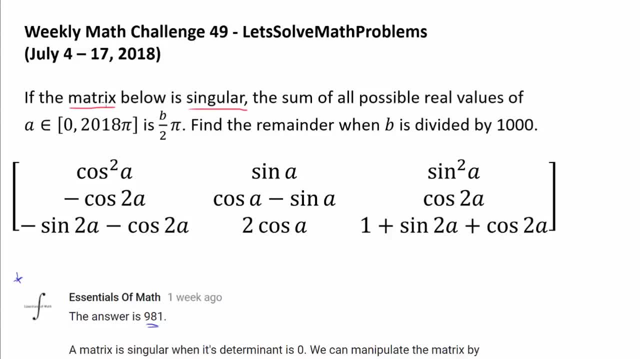 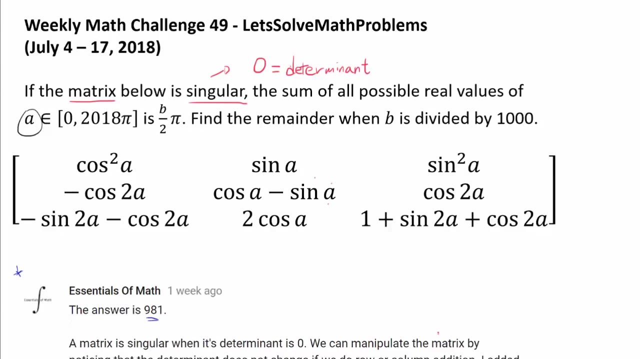 it means for a matrix to be singular. Now, this can mean many, many things, but the one we particularly care about is that singular matrix has a 0 determinant. A matrix is singular if, and only if, it has determinant of 0. So, really, what we want to find is the sum of all possible real values of A in this interval. 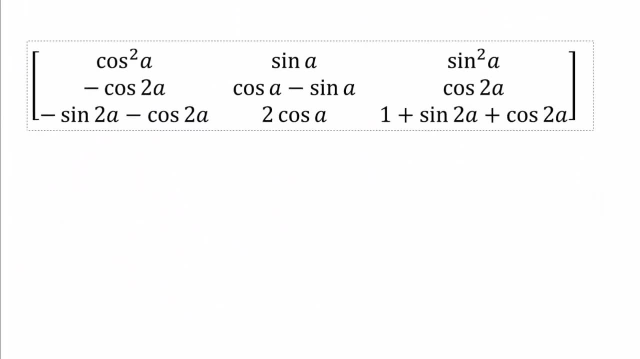 that's going to make the determinant of this matrix 0.. Now how do we simplify this? because obviously just expanding by cofactor right away is going to yield a very complicated expression that I don't want to deal with. So how can we simplify this before we actually evaluate the 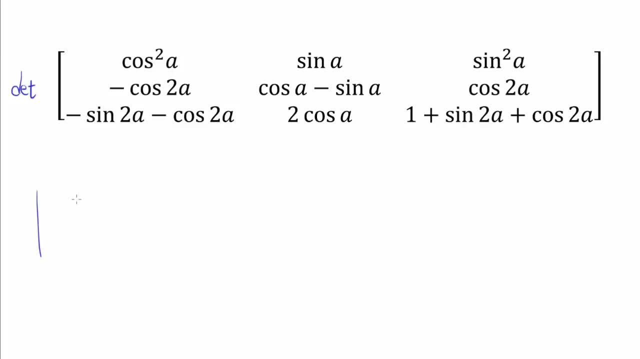 determinant. Well, you may know from your linear algebra class, or perhaps even an algebra class, that when you want to evaluate a determinant, let me just make it easy. Let's make it 1,, 2,, 3,, 4.. So the determinant in this case is: 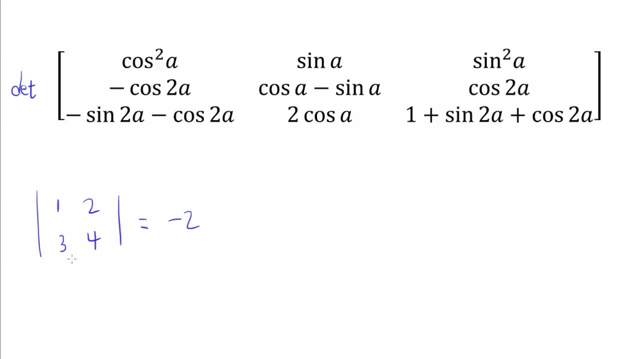 4 minus 6 or negative 2.. One operation that you can make without changing the determinant is adding a column to another column or adding a row to another row. In this particular case, if you add the first column and the second column and replace that with the first column, 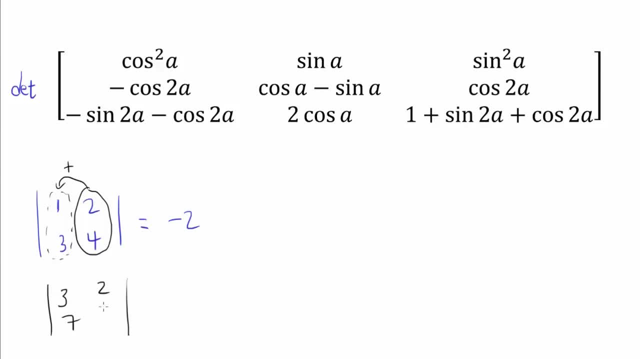 you're going to get 1 plus 2, 3 plus 4.. The second column stays the same And if you evaluate the determinant, you are going to see that it gets you the same thing. Of course I'm not going to prove it here why this works. That's for another video. But you can add: 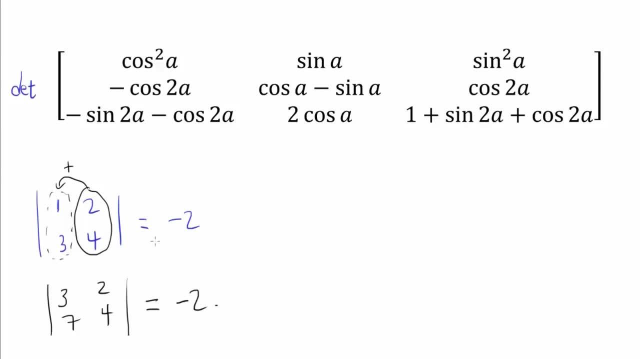 a row to a row or column to a column, like this, without affecting the value of the determinant. In fact, you can add a multiple. You can add a constant multiple of one row or column to another row or column. For example, you can multiply this column by 2 and add it to the first column, So you 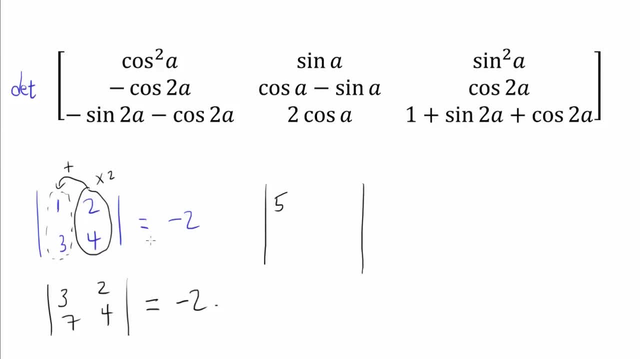 get 1 plus 2 times 2,, 3 plus 2 times 4.. So 11, 2, 4.. And your determinant is still going to stay the same. So there are various things you can do while keeping the determinant the. 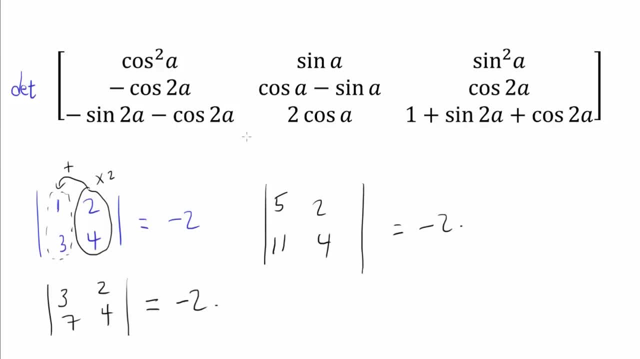 same And this is going to help us out: simplify this expression prior to actually expanding and evaluating the determinant. So what can we do to simplify this? So let's think about what operation we can make to simplify what's inside this matrix. One thing I see is that sine squared of a plus cosine squared of a is 1.. Cosine of 2a. 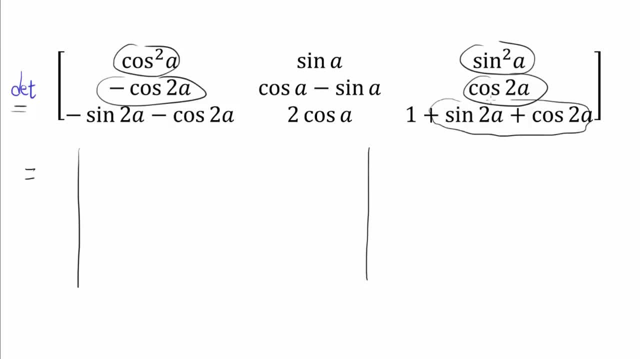 minus cosine of 2a is 0. And we have plus sine of 2a plus cosine of 2a on the right side, while we have negative sine of 2a minus cosine of 2a on the left side. So it seems. 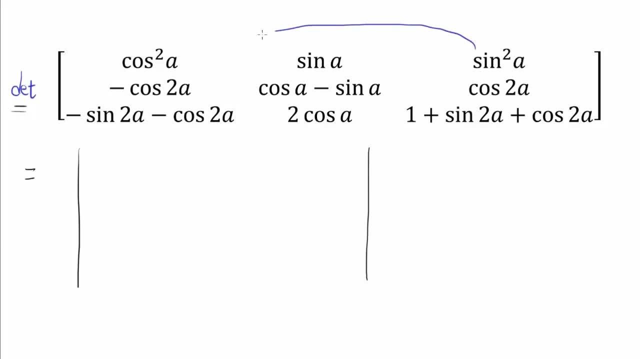 like the problem is really warning us to add the third column to the first column. So let's see what happens. As stated, this is going to keep the determinant the same. So when you add the third column to the first column, we are going to get 1,, 0, and 1.. And we are going to have sine of. 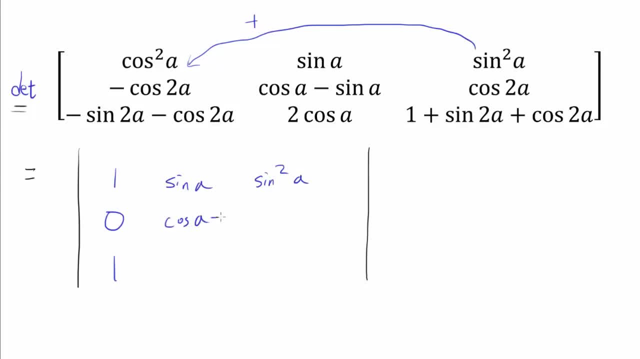 a sine squared of a cosine of a minus sine of a cosine of 2a, 2 times cosine of a 1 plus sine of 2a plus cosine of 2a. Now, from here there are many different ways of approaching. 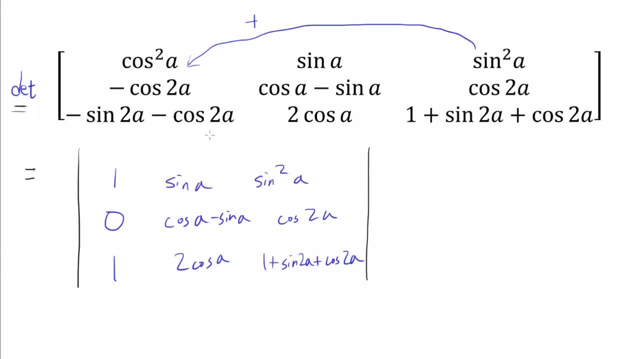 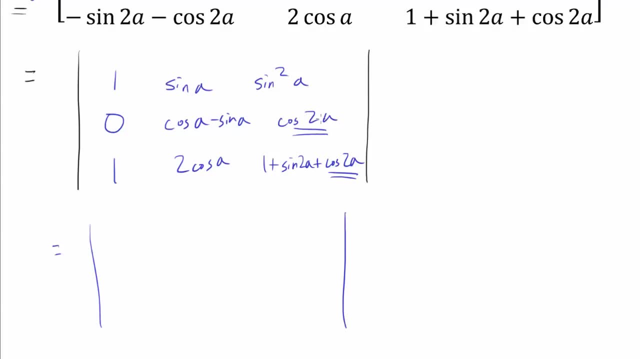 this. This is the way that I find particularly delightful. From here, let's realize that we have cosine of 2a here, cosine of 2a on this row too, And when we do 2 times cosine of a minus- this expression minus- cosine of a minus, sine of. 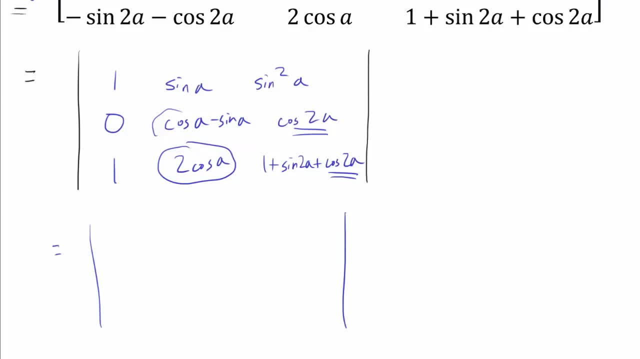 a, we are going to have cosine of a plus sine of a. Let me make that clear. So if we do 2 times cosine of a, minus cosine of a, minus sine of a, that's going to get us cosine of a plus sine of a. 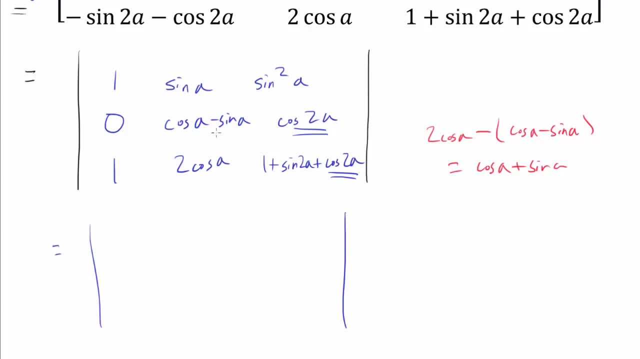 Which seems rather symmetric with the expression that we already have. So let's try it. So let's try doing this row minus this row. So we are going to start with this row. take away this row, because, cosine of 2a, we are going to cancel out and we are going to have 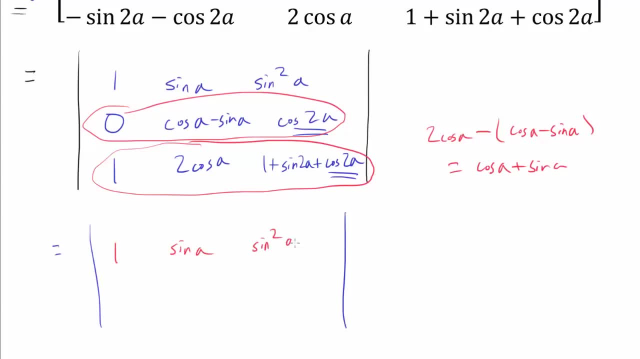 more symmetric expression. So when we do that, so sine squared of a zero cosine of a minus sine of a cosine of 2a. So when you do this row minus this row, we are going to have a 1 cosine of a plus a. 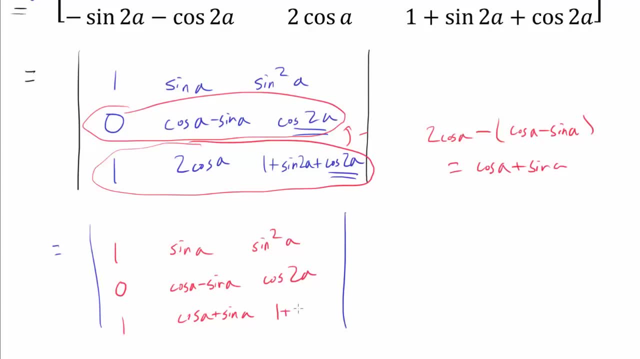 A plus a is just a êtes. A plus a equals add to 2a squared of a like that. Well done there, Because들, as we have shown, and we are going to have 1 plus sine of 2a- Now you may say where am I going with this. 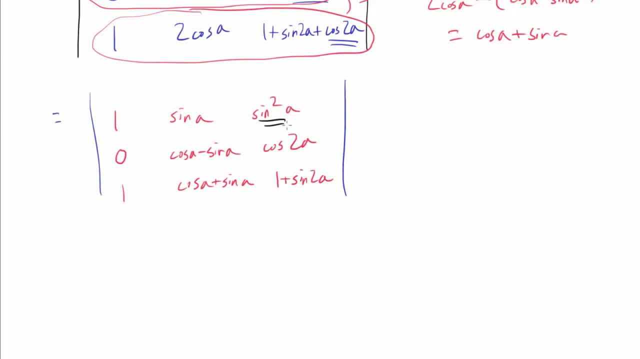 Well, look at this: You have 1 sine of a sine squared of a and we have 1 cosine of a plus sine of a, and this may not be immediately obvious, but realize that 1 plus sine of 2a is cosine of a plus sine of a squared. 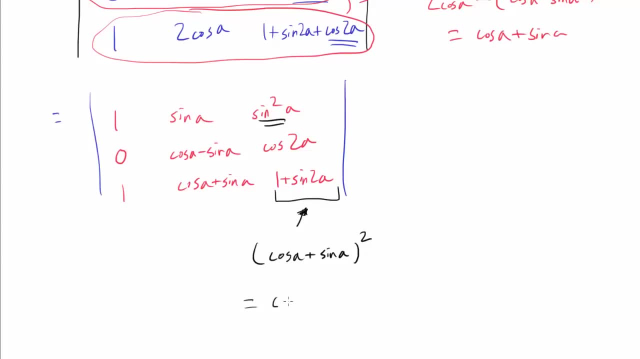 because cosine of a plus sine of a squared is cosine squared of a plus 2 times cosine a sine a plus sine squared of a, and cosine squared of a plus sine squared of a is 1, and 2 times cosine of a times sine of a is sine of 2a. 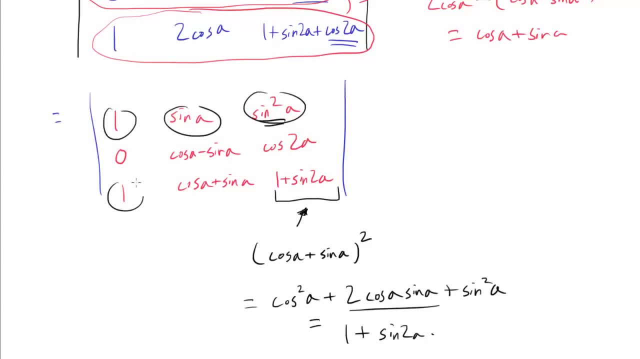 So we have 1 sine of a times sine squared of a 1 cosine of a plus sine of a cosine of a plus sine of a squared. and this may remind you of Vandermonde determinant, Vandermonde Andermonde Determinant, one of the more famous determinants in linear algebra. 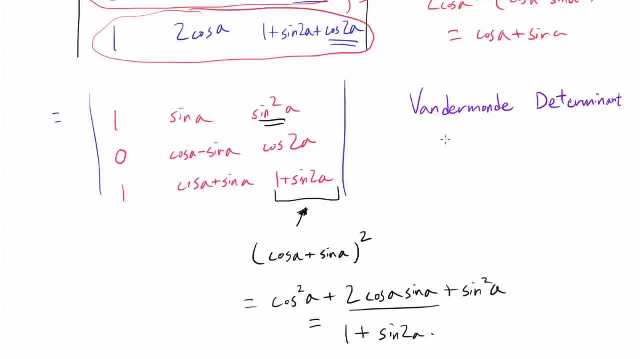 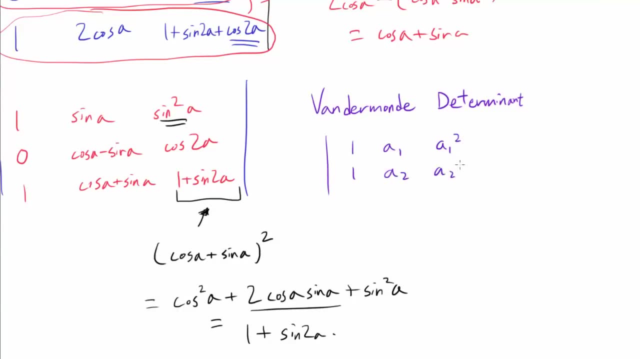 determinant which state for 3 by 3 case that determinant of 1 a sub 1 a sub 1 squared, 1 a sub 2 a sub 2 squared, 1 a sub 3 a sub 3 squared is going to be a sub 3 minus a sub 2. 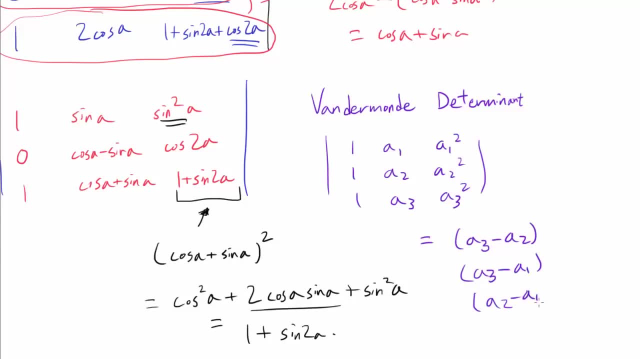 a sub 3 minus a sub 1 times a sub 2 minus a sub 1.. So this is the determinant of this matrix And in fact you can generalize this to a n by n matrix And in fact I may make a video on. 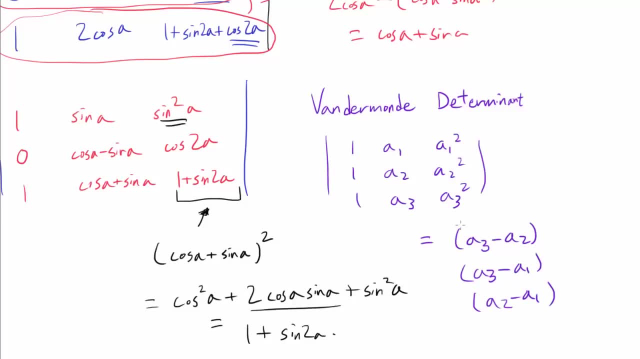 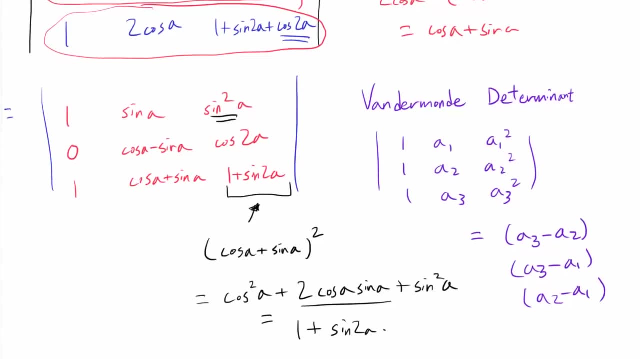 Vandermonde Determinant and giving you a proof of why this works. There's a very elegant proof that you can use using factor theorem for polynomials, But that's again, that's for another video. But you may realize that maybe we can make a Vandermonde Determinant out of this. 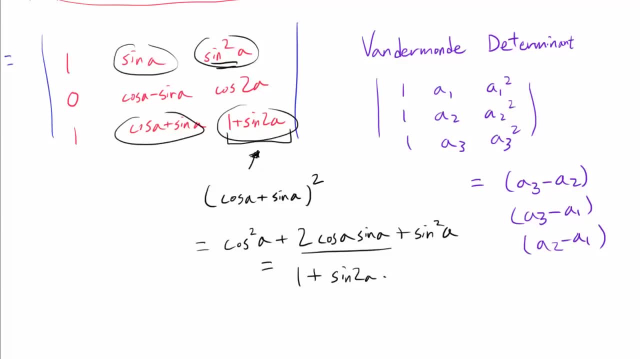 because we have something, something squared, something, something squared. So let's think about how to modify this Second row, if possible, to get the Vandermonde Determinant. And we see that cosine of 2 a, cosine of 2 a is cosine squared a, minus sine squared a. So it looks like when we add these: 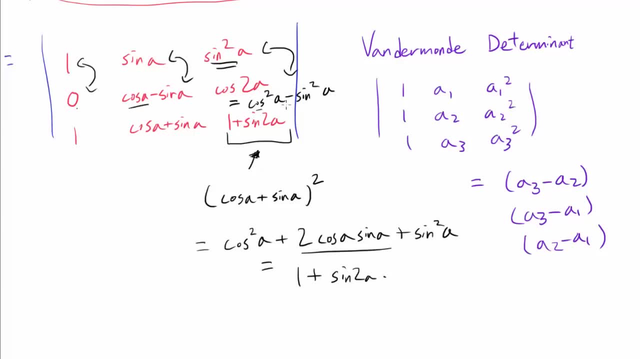 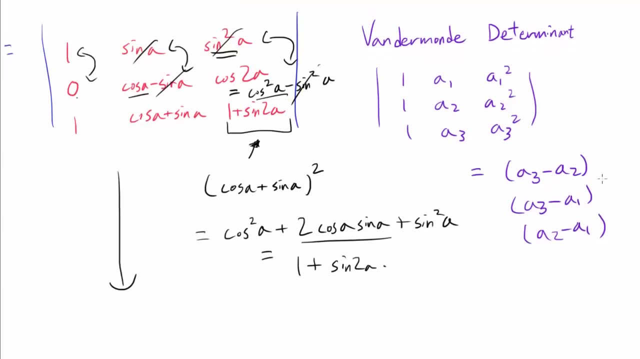 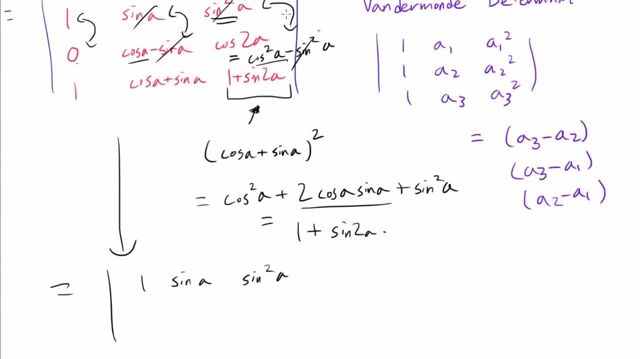 two rows. we are going to have one cosine of a, then cosine squared of a, because the sine of a's are going to cancel out and sine squared of a's are going to cancel out. So let's do so. So when we, when we do that, we are going to get one sine of a, sine squared of a. when we. 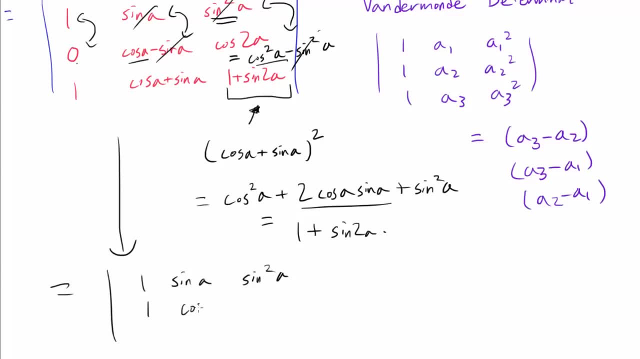 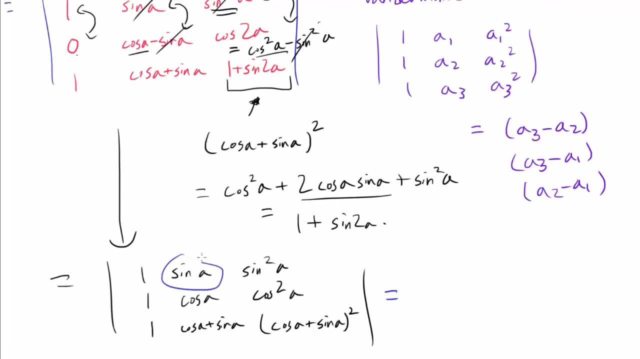 add the first row and the second row, we get one cosine of a, cosine squared of a, one cosine of a plus sine of a. then finally, we know, this is cosine of a plus sine of a squared. So we here we have it, here we have Vandermonde, Determinant. In this case, a sub one is sine of a, a sub two is cosine of a. 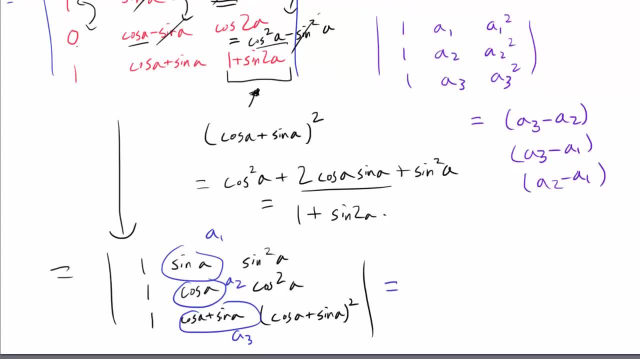 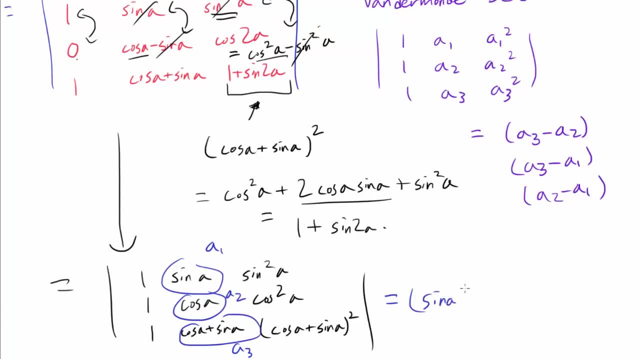 and a sub three is cosine of a plus sine of a. So we know this determinant is going to be a sub three minus a sub two or sine of a times a sub three minus a sub one, or cosine of a times a sub two minus a sub one, or cosine of a minus sine of a. 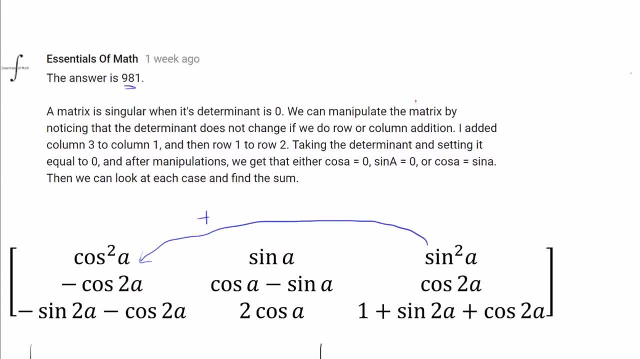 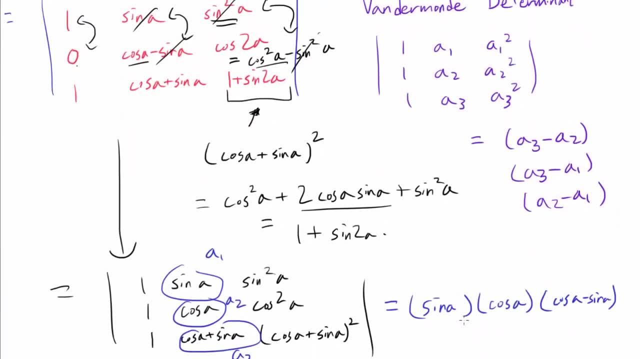 And once again, because we want the matrix to be singular. we want the matrix to be singular, we want the determinant to be zero, So we are looking for the values of a where this thing is zero. So we want sine of a to be. 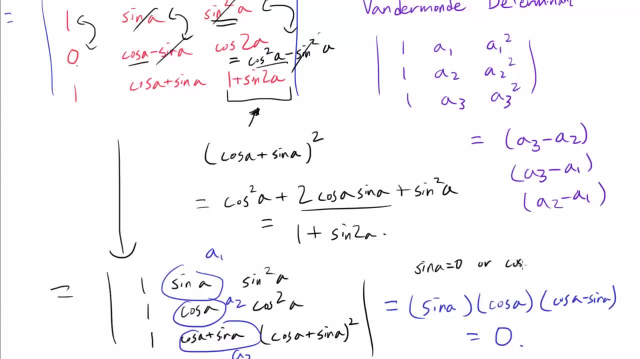 zero. So we want sine of a to be zero, or cosine of a to be zero, or, finally, we want cosine of a minus sine of a to be zero, or cosine of a to be equal to sine of a. So these are three different. 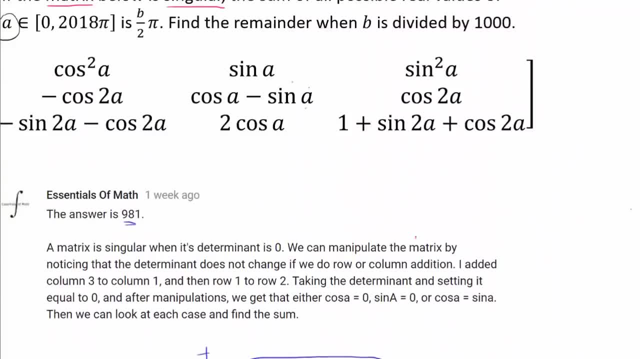 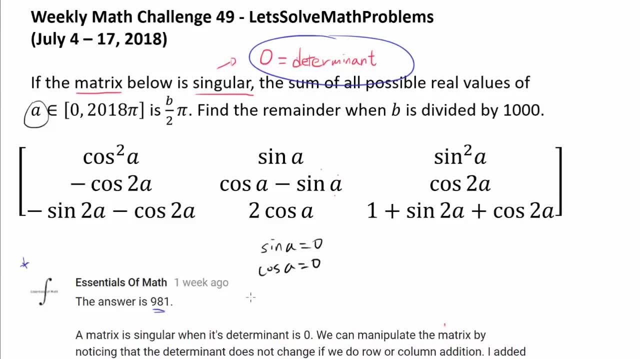 cases we have to care about. So let's go all the way back up. So we know, so we care about the cases where sine of a is zero, cosine of a is zero And the case where sine of a is equal to cosine of a. So let's analyze these And we are going to find the sum of all possible values of a that 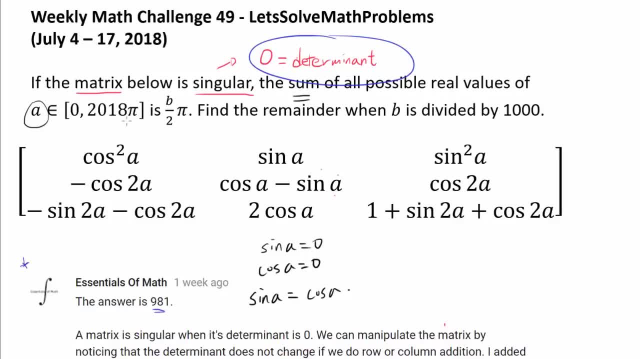 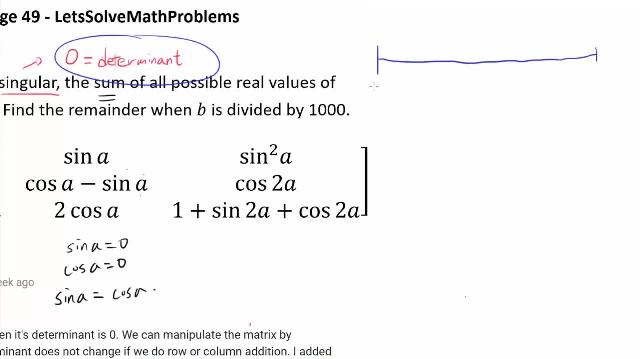 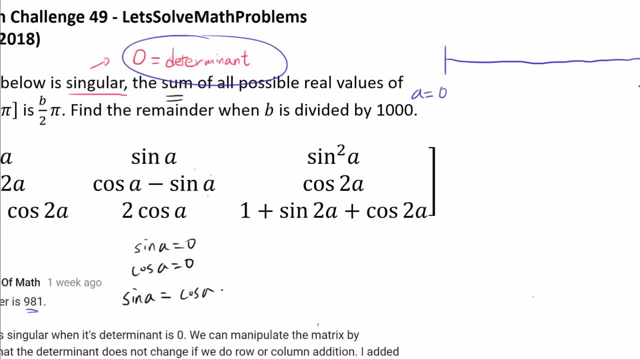 satisfies this in the interval from zero to 2018 pi, And this is how I'm going to break this question apart. So we are looking for all the possible values of a, from zero all the way to 2018 pi, And, obviously, even if a equals to zero satisfy one of our equations- it does, in fact, but we 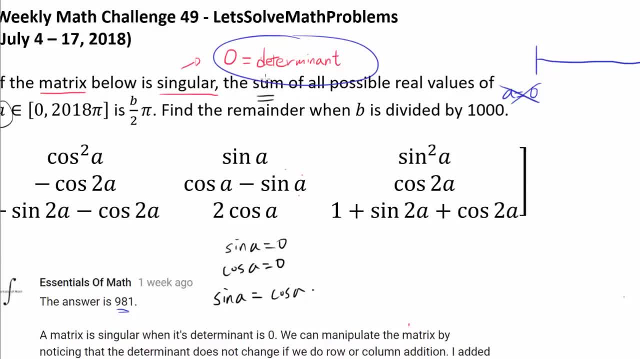 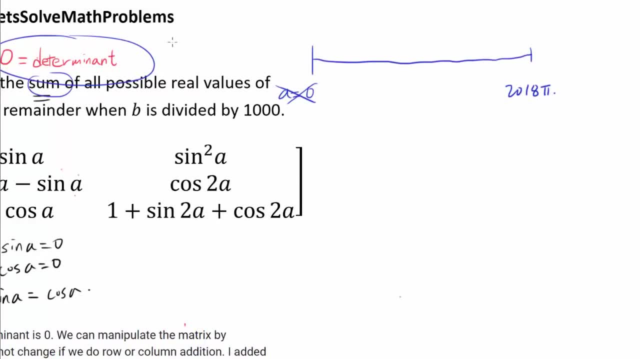 really don't care about a equals to zero, because we are finding the sum. a equals to zero is not going to change the value of the sum, So we don't really have to care about that. So one way of breaking the sound is to consider the interval from zero to two pi, where we exclude the zero and include the two pi, because once 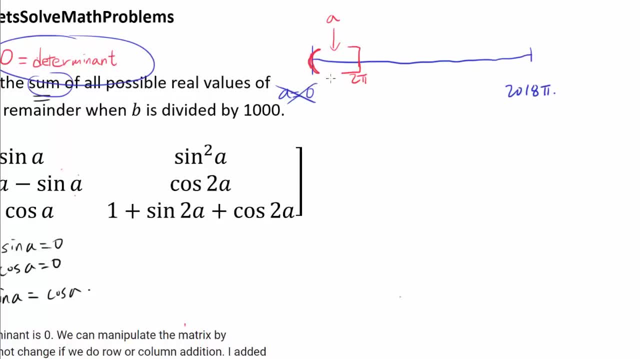 we know all the possible values of a in the interval from zero to two pi, not including zero, then we know. we know how to find all the values away from two pi to four pi, excluding two pi, because sin and cosine each has a period of two pi. So if some value in the first interval like pie, 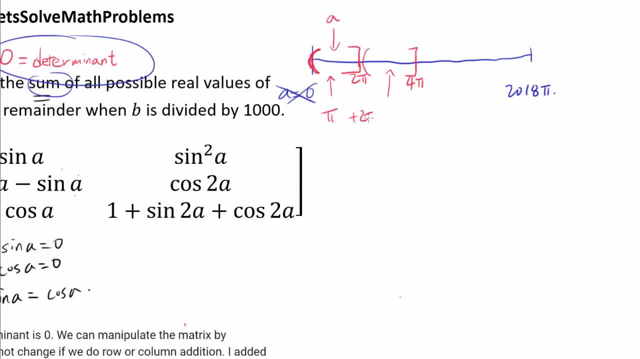 set one of our equations, then you know pi plus 2 pi or 3 pi is going to be in the second portion satisfying one of our equations. so once we know it for 0 to 2 pi, then we know it for 2 pi to 4 pi. 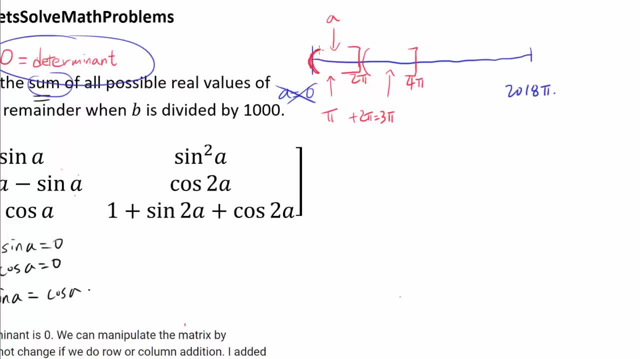 and so on. and you may say: why am i? why am i doing this? why am i not including 0 here, not including 2 pi here, and so on? well, if i include 0 here and include 2 pi here, then we're counting 2 pi twice. 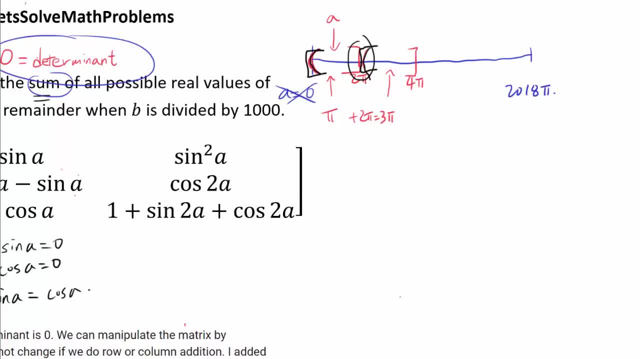 because it's been counted for the first interval and it's been counted for the second interval. so i'm doing it like this: open on the left, close on the right, so each number gets counted once. enough about that. now let's actually try to find the values of a from 0 to 2 pi, excluding 0. that 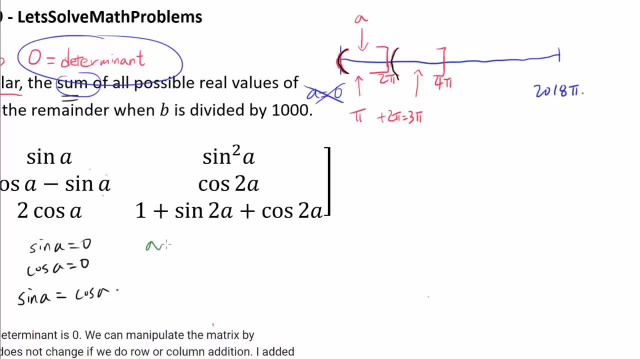 satisfy one of these equations: sine of a is equal to 0 gets us the solution: a equals to pi or 2 pi. cosine of a 0 gets us the solution: a is pi over 2, 3 pi over 2 and, of course, sine of a is equal to cosine of a. add pi over 4 and 5 pi over 4.. So what's the sum, What's the? 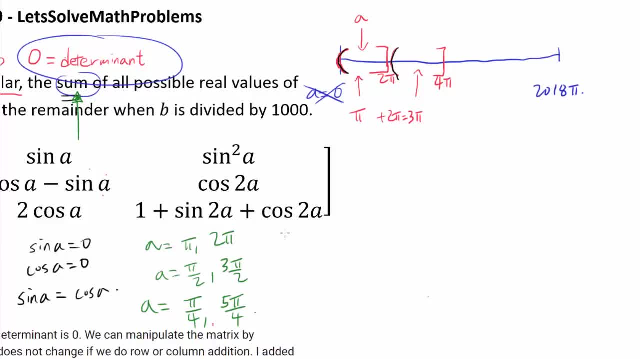 sum of all possible values of a In the first interval, pi plus 2 pi- is 3 pi. pi over 2 plus 3, pi over 2 is 2 pi. pi over 4 plus 5 pi over 4, that's 3 pi over 2.. And when you add up every 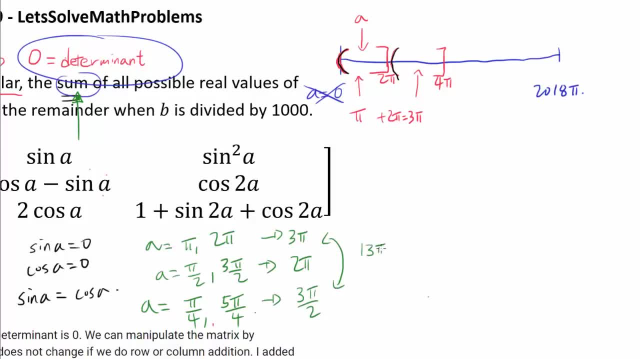 single one, that's 5 pi plus 3 pi over 2, or 13 pi over 2.. So for the first interval we get the sum of 13 pi over 2.. Now what about the second interval? Well, in the second interval, each of 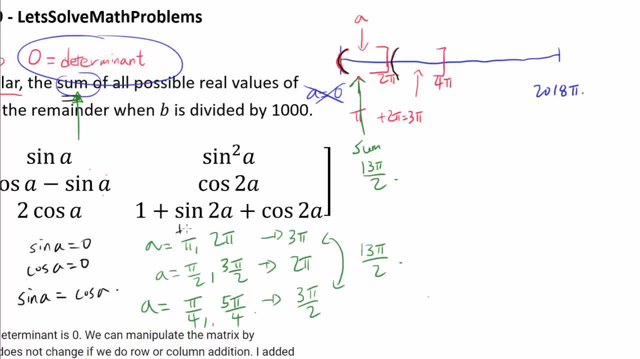 these solutions. so each of the six solutions is going to be incremented by 2 pi. Each of them plus 2 pi is going to be the solution for the second interval, And we see that that's going to be the same thing as 13 pi over 2, plus how many 2 pi's, 6 of 2 pi's, so 12 pi. So the sum for the 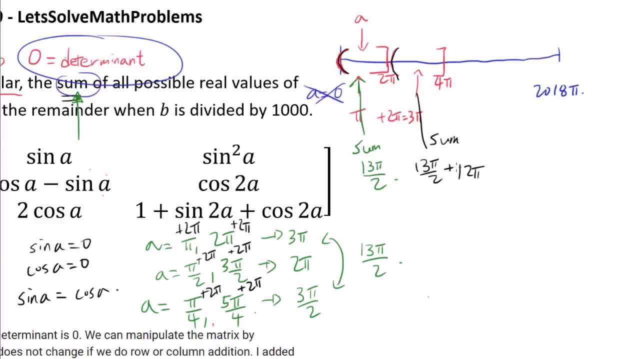 second interval is going to be the sum for the first interval plus 12 extra pi's And we see that from 4 pi to 6 pi we are going to have 13 pi over 2 plus 24 pi adding another 12 pi. 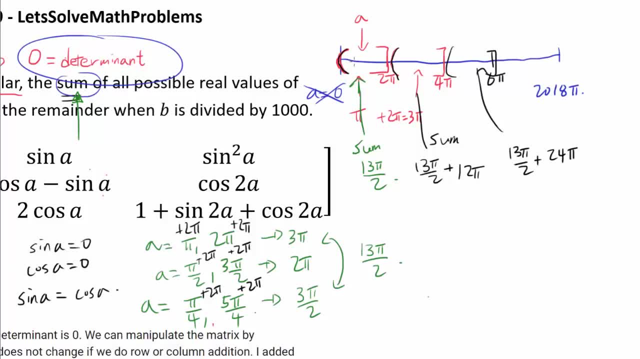 So we have this arithmetic sequence, And how many intervals do we have? Well, each interval is going to be the same thing as 13 pi over 2.. So we are going to have 13 pi over 2 plus 24 pi. So we have this arithmetic sequence. And how many intervals do we have? Well, each. 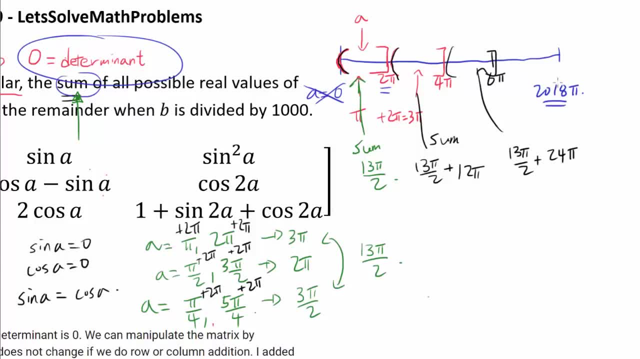 interval is of length 2 pi, and we are going all the way to 2018 pi. So we have 1009 intervals. we have 1009 intervals or 1009 terms in the arithmetic series, And all we want to do is add. 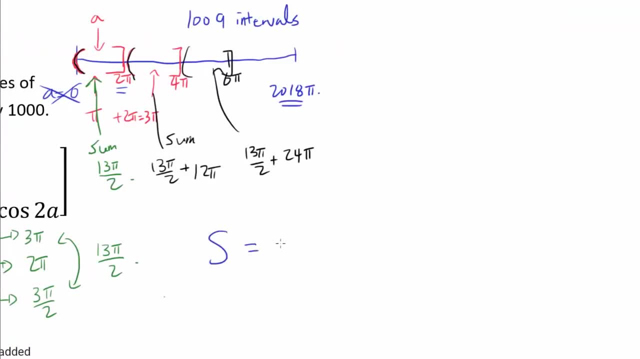 them up And, as you know, the sum for the arithmetic series is n over 2 times 2 times a sub 1 plus n minus 1 times t, where a sub 1 is the first term, n is the number of terms, in this case 1009.. And d is the common difference. That's the common difference And of 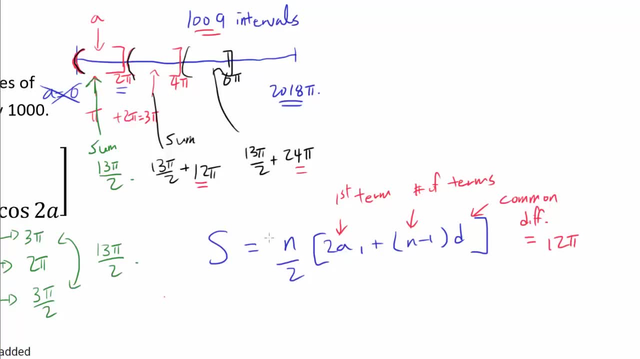 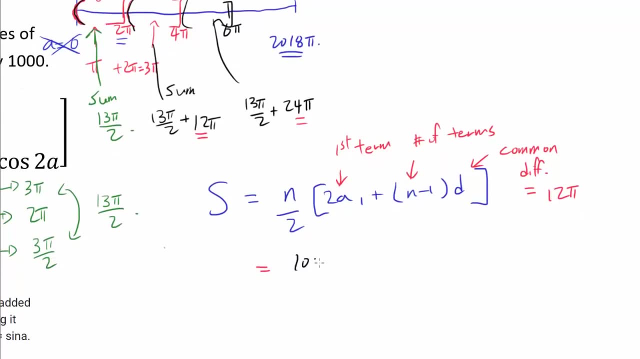 course, common difference in this case is going to be 12 pi. That's what we are adding each time. So what's the value of our sum n is 1009.. Once again, so 1009 over 2 times, 2 times a sub 1,. 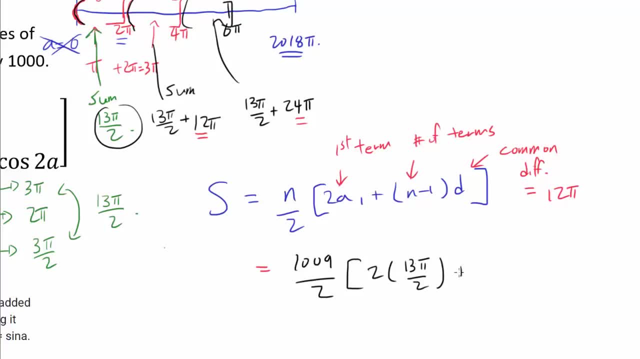 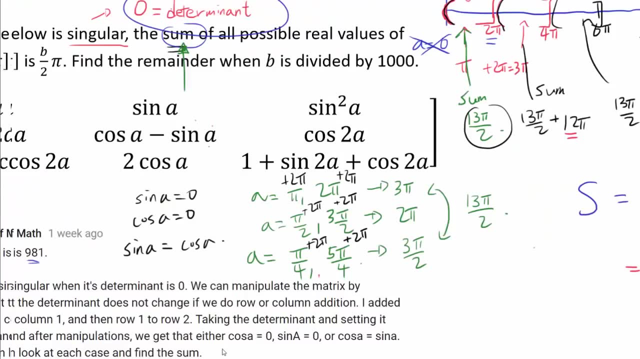 which is 13 pi over 2,, 13 pi over 2, plus n, minus 1,, 1008.. times d or 12 pi, And what do we want to do? We know this sum is b over 2 pi and we want to. 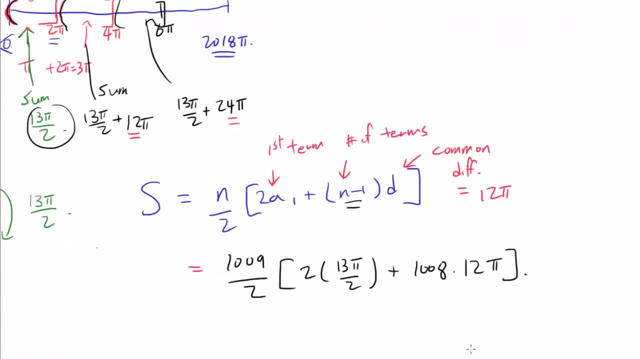 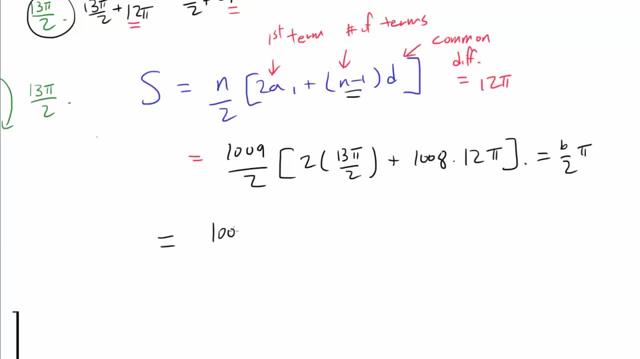 find b mod 1000.. So we know this thing is equal to b over 2 pi. So let's try to simplify this just a bit. So we have 1009 over 2, and we have 13 pi, and we also have 1008 times 12 pi. So we